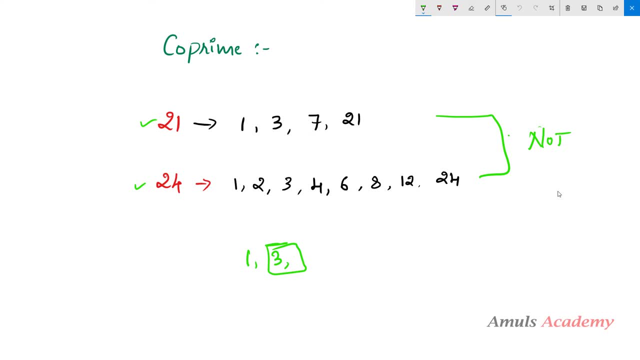 Hello guys and welcome to Python programming tutorials by Amuls Academy. and in the previous tutorial we discussed about the co-prime numbers, and a number can have multiple co-prime numbers. If i want to print that, then how to do that, so i will explain you about that in this program. 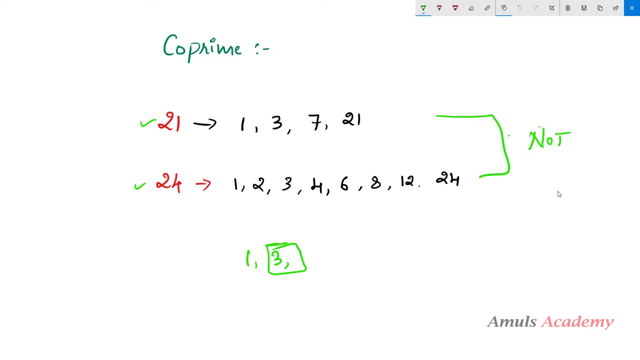 So how to print co-prime number of a particular number in a specific limit? ok, so co-prime number is nothing, but if the gcd of two numbers is 1, then that two numbers are co-prime numbers. So if i take number as 12, so i want to find out all the co-prime number of 12.. 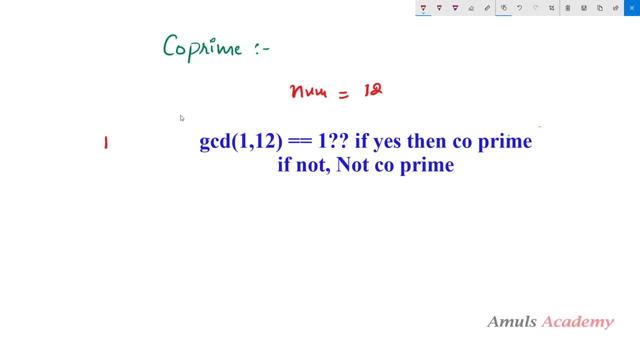 So first i can take 1, so i can check 1 and 12, so 1 is the co-prime of 12.. You can write down the factors and you can check. so the factors of 12, divisor of 12. 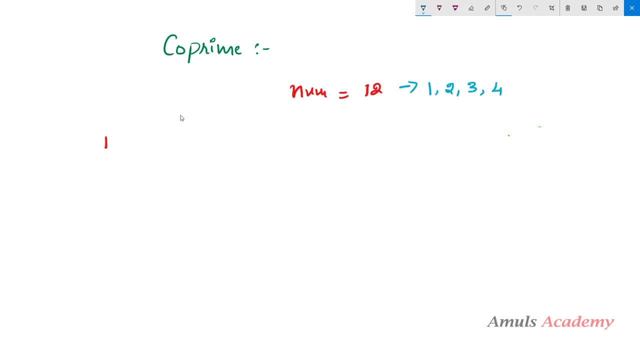 is 1.. 1,, 2,, 3,, 4,, 0,, 5,, 6,, 12.. So i can check the factor of 1 is 1,, so the common is 1.. So gcd of 12 and 1 is 1, that means 1 is the co-prime number of 12. ok, 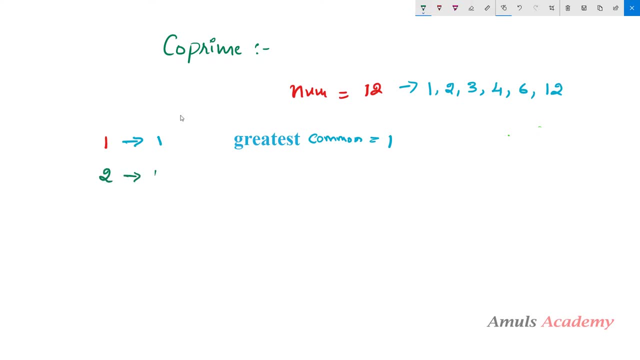 So next i can check with the 2. ok, so divisor is 1 and 2,, so common is 2.. ok, so gcd of 12 and 2 is 2, so 2 and 12 are not co-prime numbers. no, 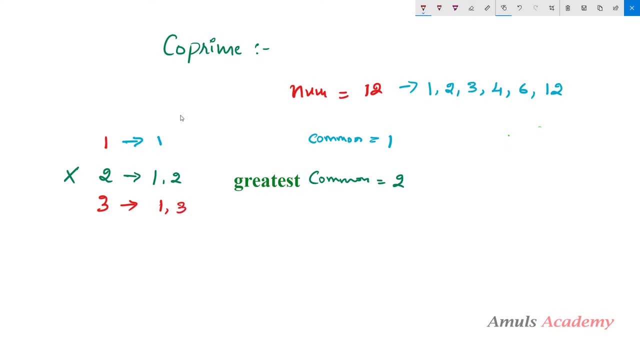 And i can check with 3. ok, 1 and 3, so here common is 3, so 12 and 3 are not co-prime. i can check 4.. 1, 2 and 4.. So common is 4, gcd of 4 and 12 is 4, so 12 and 4 are not co-prime. 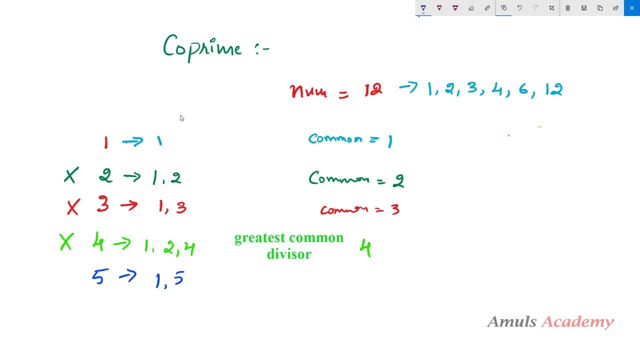 So i can check for the 5, 1 and 5. ok, So common is 1, so 5 and 12 are the co-prime numbers like this i can check. So till now, 1 and 5 are the co-prime of 12, there are many. 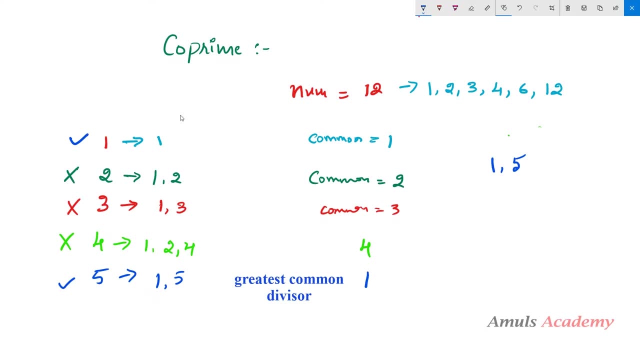 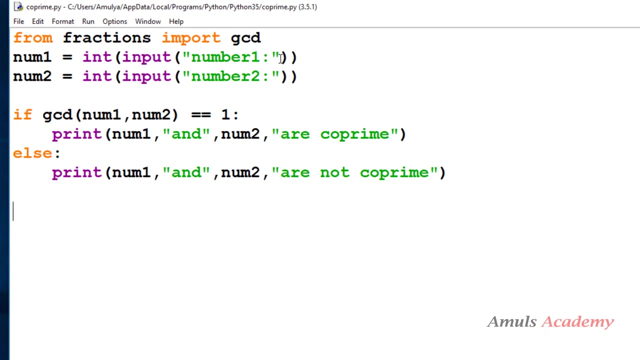 Like 7, 11, right? So we can print all the co-prime number in a particular limit of a specific number. So for that we will write the program today. So this is the previous program. so here we want a single number, so we don't want another. 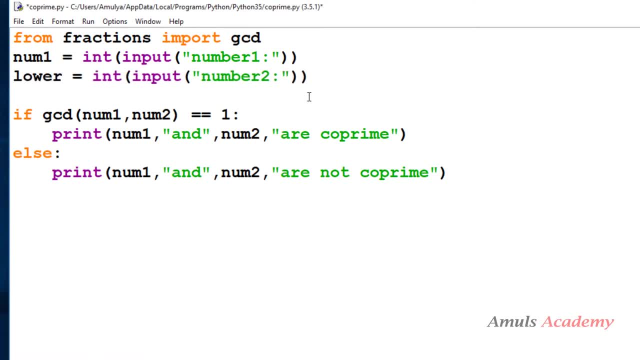 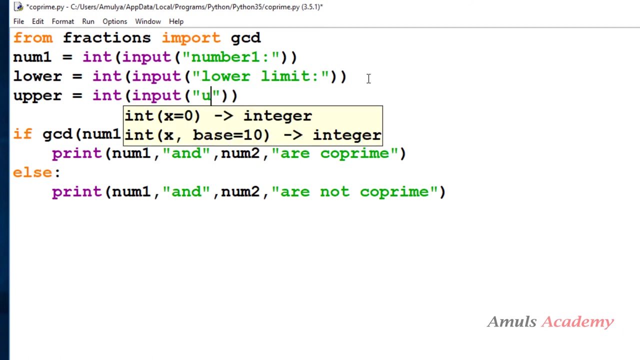 number. here we want limit, lower limit and upper limit. That is, from where to where. You want the co-prime number of specific number, from where to where. that is the lower limit and upper limit. ok, so first i need to take a number and lower limit and upper limit. 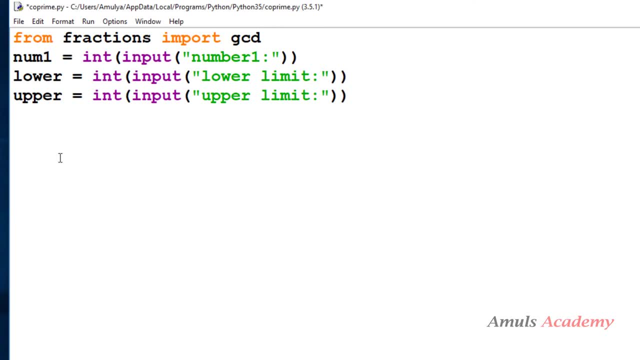 So here, first of all, Ok, I will take for loop lower to upper plus 1.. So i want to go through each element of this lower limit to upper limit. If i mention 1 to 10, lower limit is 1, upper limit is 10.. 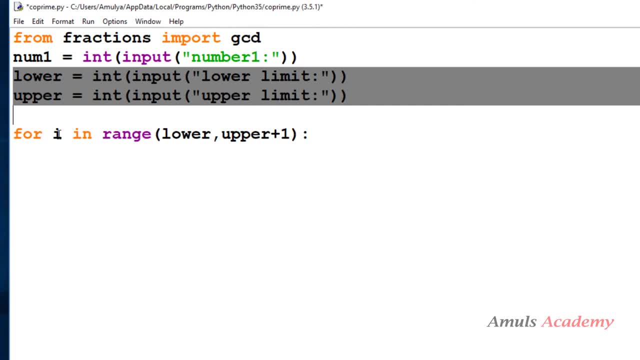 First i want to go through 1,, 2,, 3,, 4,, 5,, 6,, 7,, 8,, 9,, 10, right? So that's why here i took the range as upper plus 1.. 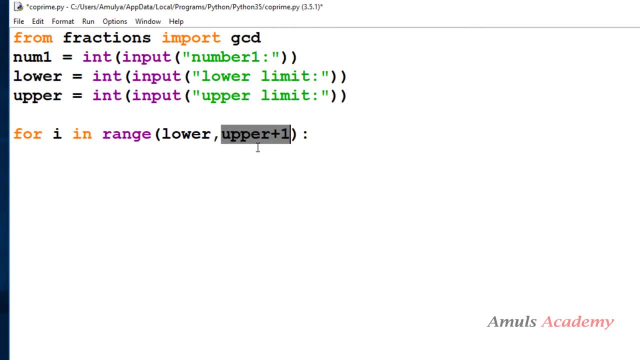 Because in the range function the end or this part is exclusive. that's why i need to take upper plus 1.. If i want 1 to 10, then i need to take here 1 to 11. ok, And here i will check gcd of the number 1, so that is the particular number and i is 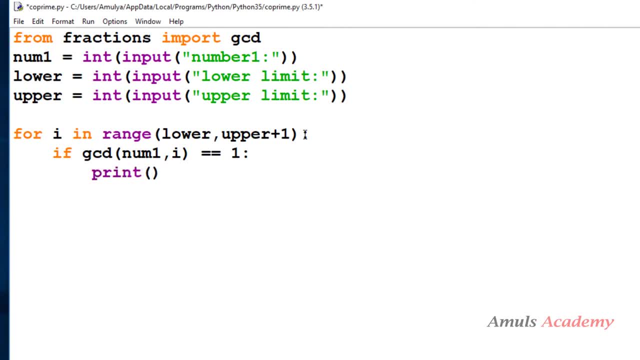 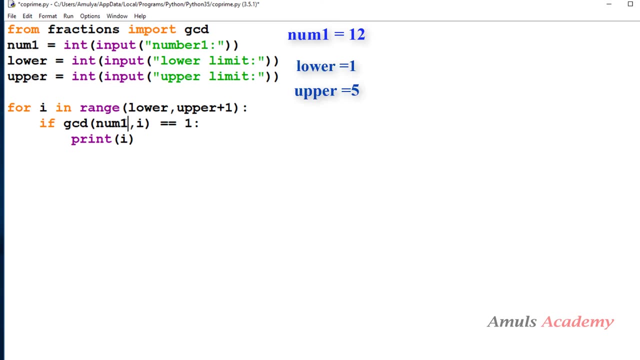 equal to 1, print that number. Ok, i else do nothing. i don't want to do nothing, So this is nothing. but here i will check the gcd of given number. for example, if you enter 12, so i need to check 12 and gcd of 1, if it is 1,. if yes, then i will print that number. 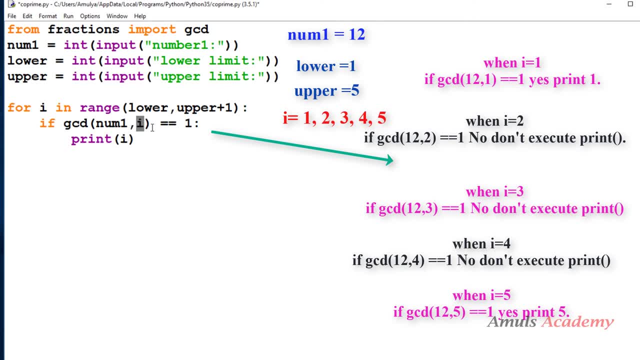 if not, i will go to the next number. i will check 12 and 2. ok, next i will check 12 and 3,, 12 and 4,, 12 and 5,, 12 and 6,, 12 and 7,, 12 and 8..